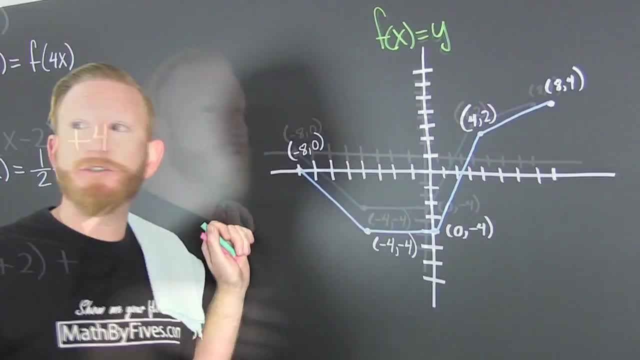 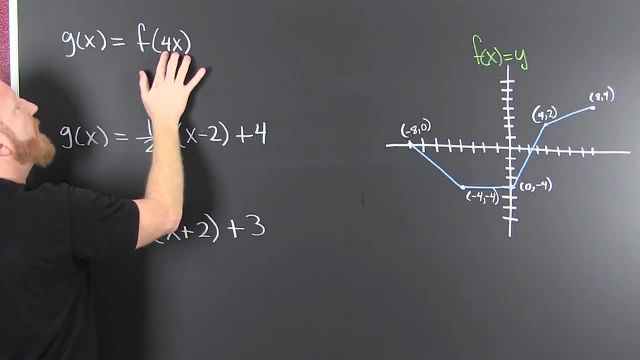 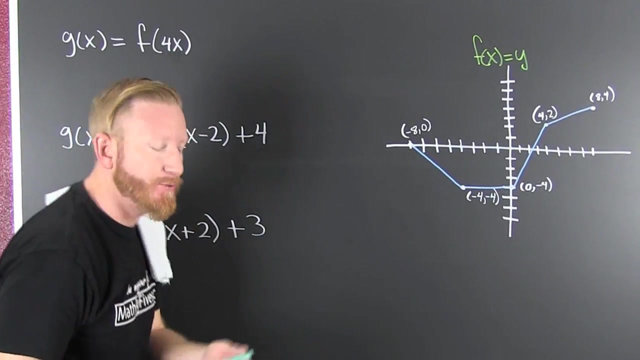 looks like this. We are going to dilate and translate this guy. First let's just look at the x's Boom. That means I'm going to take my new function g of x. It's going to have four times whatever x was What. That doesn't do what you think it does, That's. 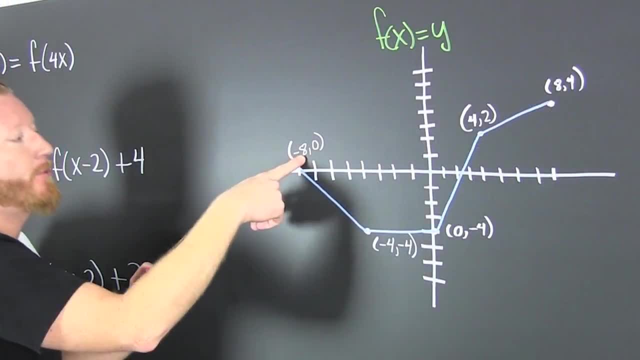 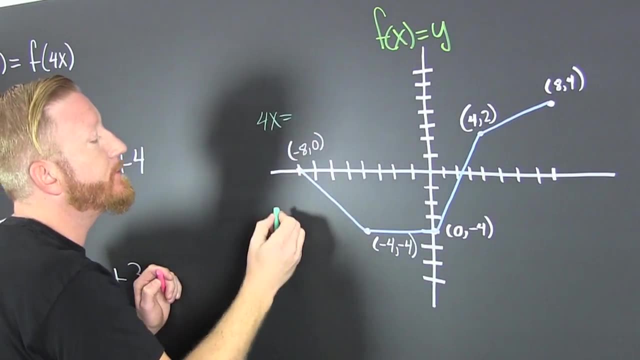 a shrink. You need a shrink. What are we doing? We're taking all of our x's, and 4x is our new x. So then 4x is equal to a minus 8.. Great, Wait, What's our new x? Our new x is going. 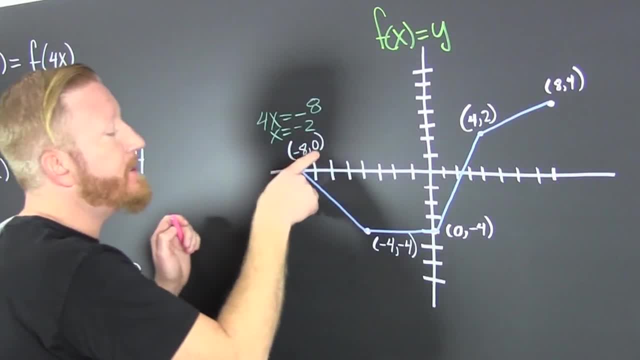 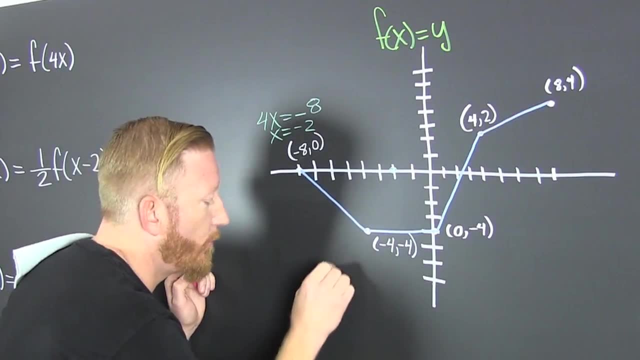 to be a minus 2.. This is shrinking things. So minus 2, 0 is going to be on there. Minus 2, 0 is on there. Then what? Here, 4x is equal to a minus 4.. Sure, because that's my x value. 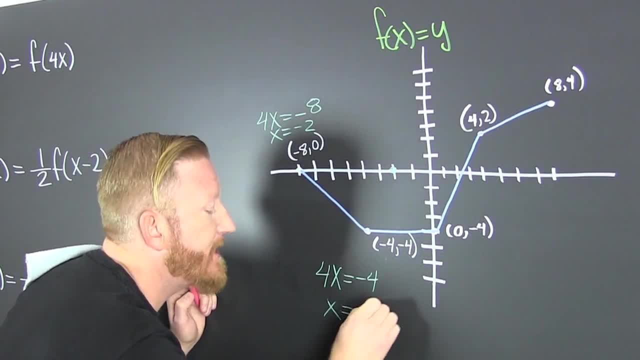 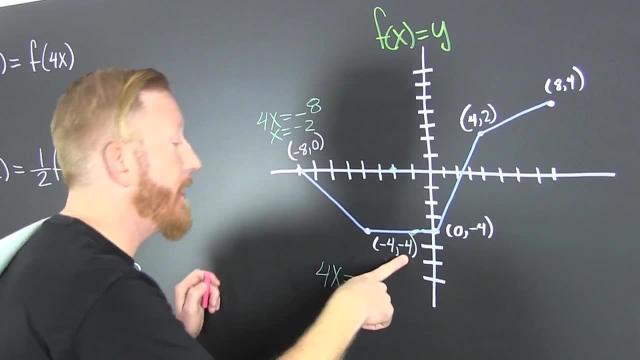 So what's my new x value going to be? My new x value is going to be a minus 1.. Fine, That's it. So minus 1, 4.. Did I change the y? I didn't. That says nothing about y We're talking about. 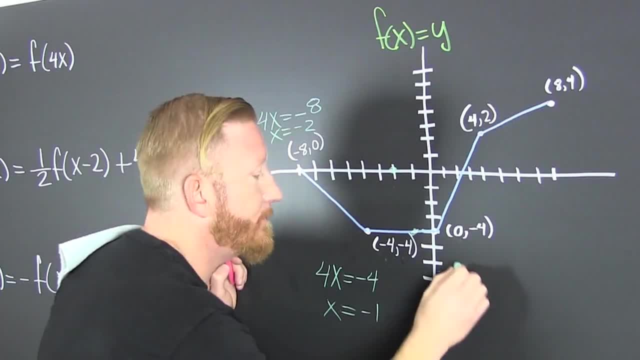 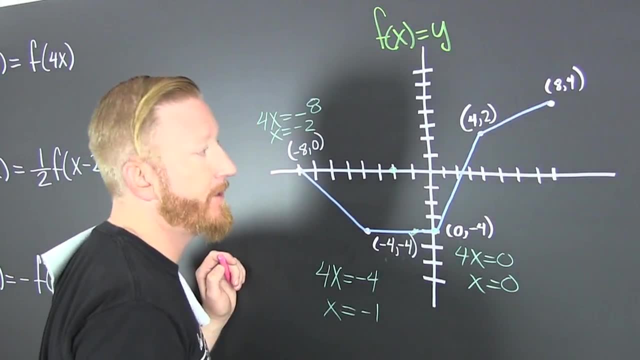 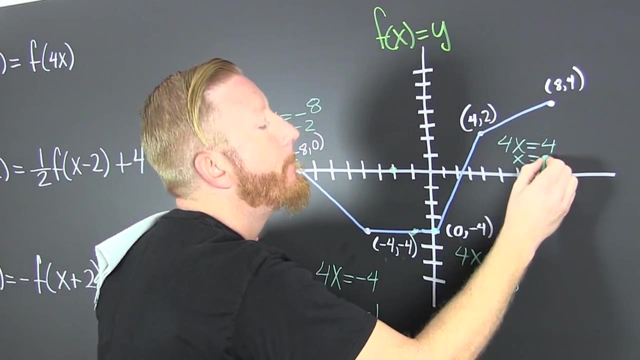 x. Yeah, So here 0. Boom 4x is equal to 0.. So x turns out to be 0.. That point remains on there. This one, 4x is equal to 4.. So then x is equal to a 1.. So then x is 1.. Boom, Didn't. 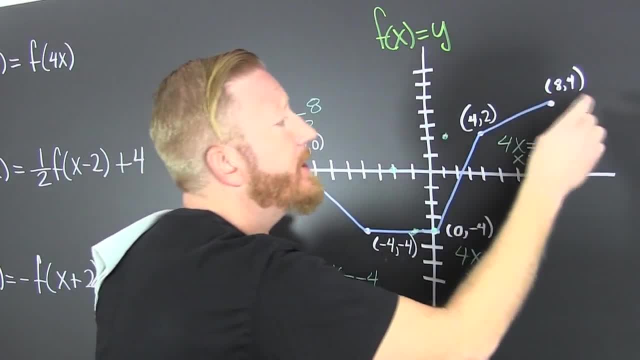 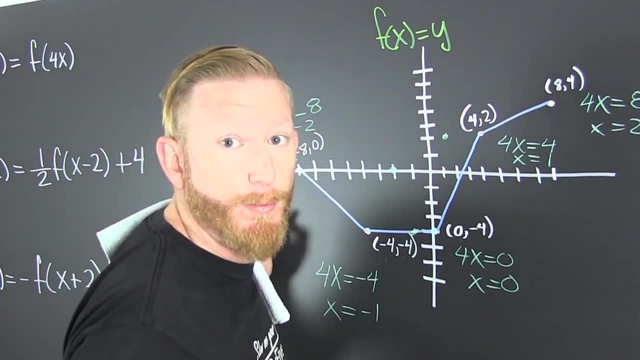 change the y, Still a 2.. So now I'm looking here: Here 4x is equal to 8.. And then x turns out to be 2.. We're finding our new points with this function notation. We're in the interior of the function. 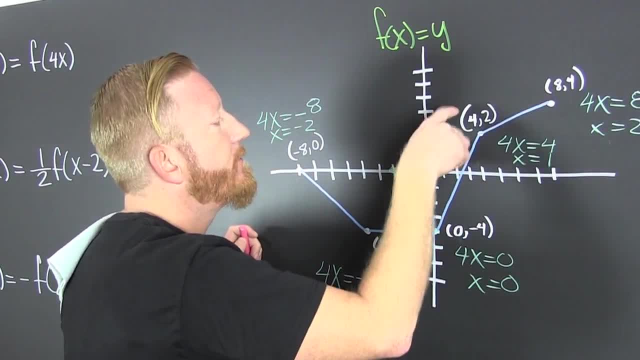 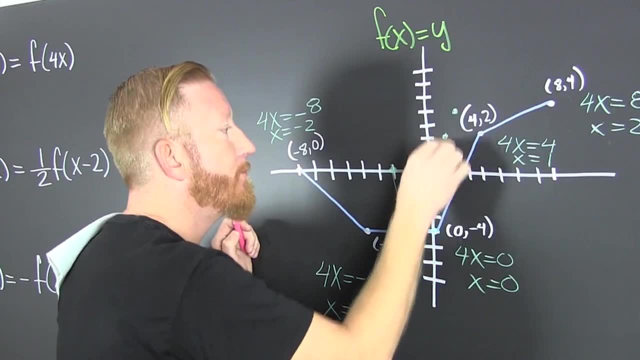 So we're looking at x, And here our new x is 2.. So 2, 4 is on there, 2, 4 is on there, And then we can make that graph: Boom, Boom, Boom Boom, And then that's what g of x looks. 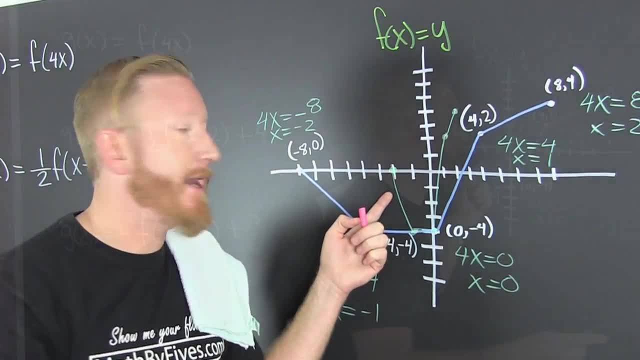 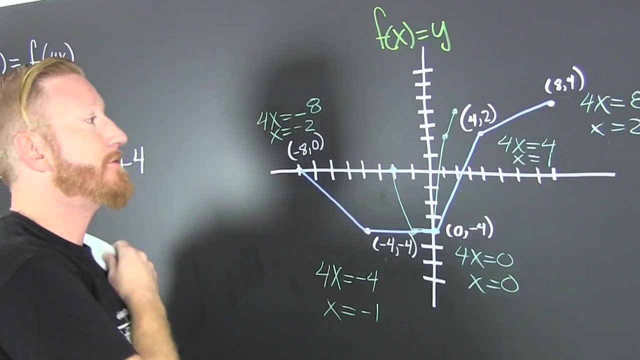 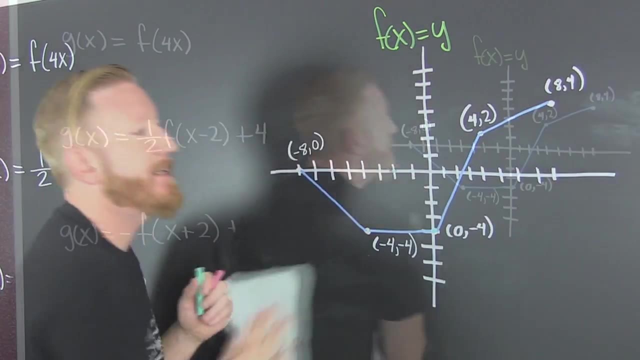 like when g of x is equal to f of 4x. That guy, Let's go get another one. I'm going to give you a second to write that down: 1.. So let's get rid of this. Next, In the next example. 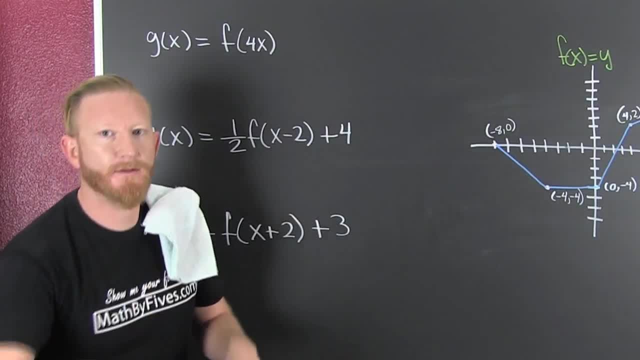 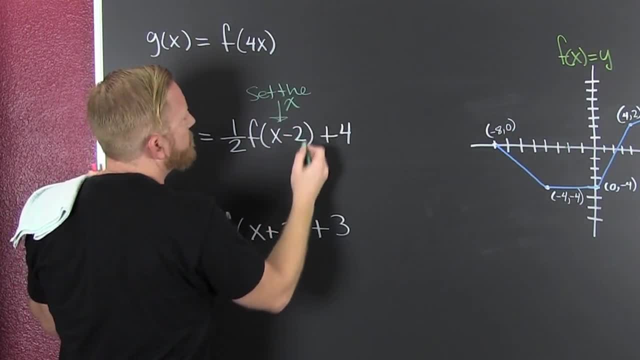 1. 0. 1. 0. 1. 1. 1. 0.. 1. 1. 0.. 1. 0 0. 0.. Day 2, both sides of the graph, is 70%. 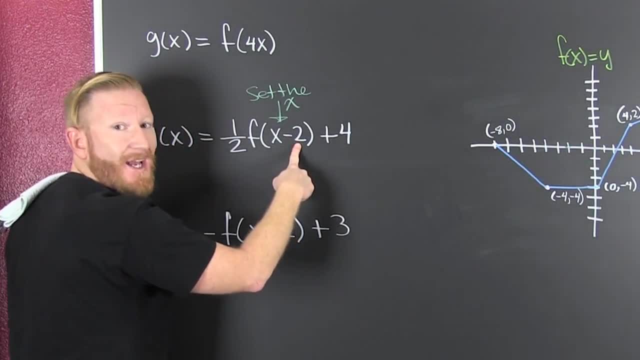 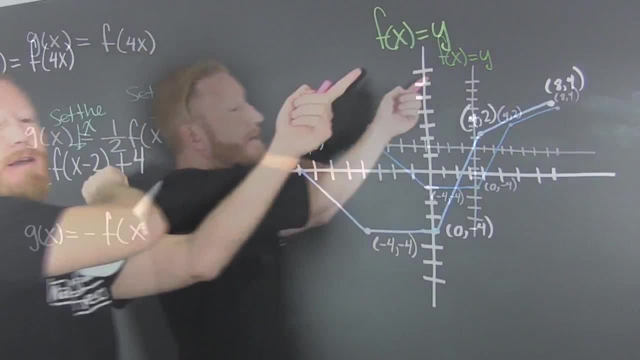 Was that time long enough? Set all the x's equal to and x-2. And find the new ones. I guess you could short step it and add 2 to both sides, but whatever, Now f of x is the function formal known as y. That's what I was trying to instill, right there. 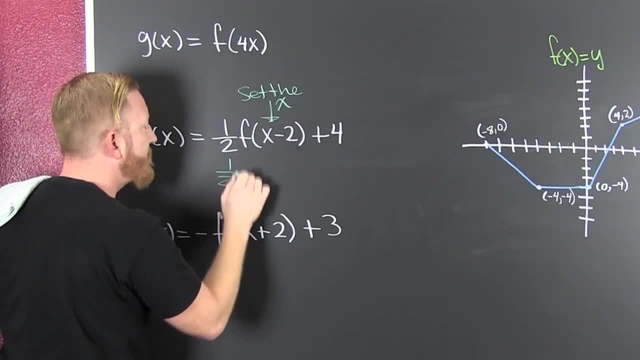 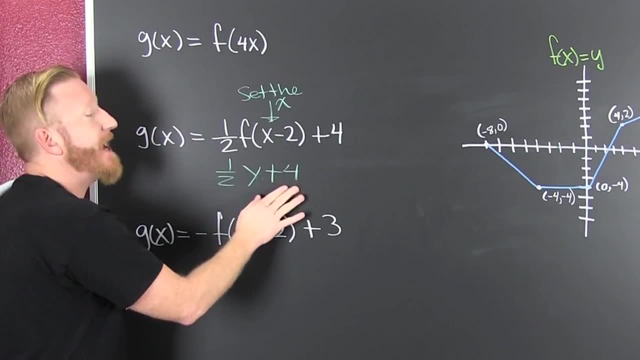 So what are we gonna do? We're going to take y, Sure, So we're going to take half of y and then add 4 to it. Let's go and get to it. Let's find our new x. x minus 2 is equal. 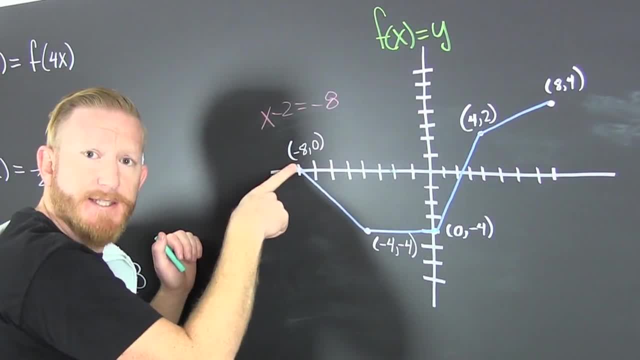 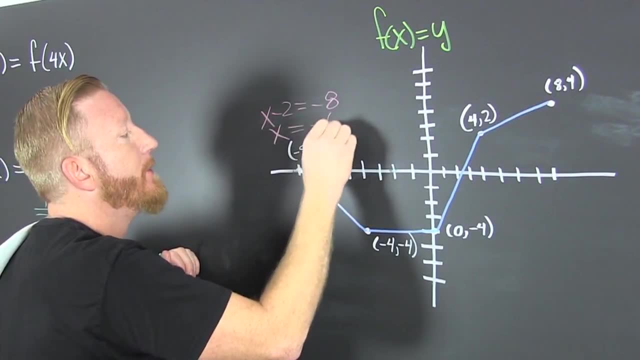 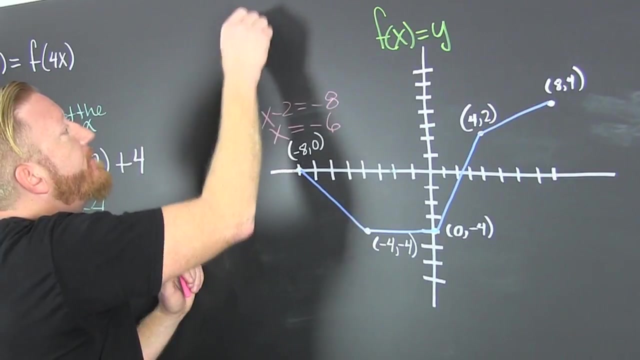 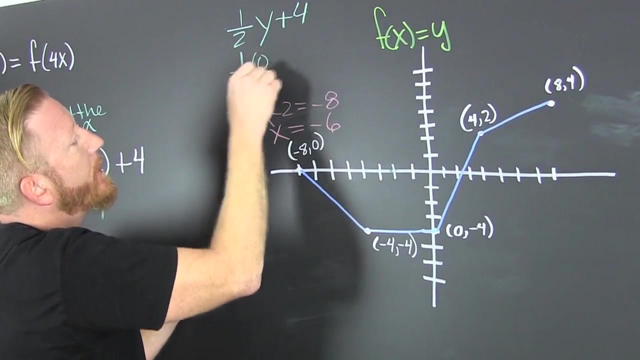 to a minus 8.. Great, We're translating this point so we can change this function into g. So then g. I see my x is going to be a minus 6.. But wait, there's more. Since I have 1 half y plus 4, I can go and I can do that there. That's 1 half 0 plus 4, which is equal. 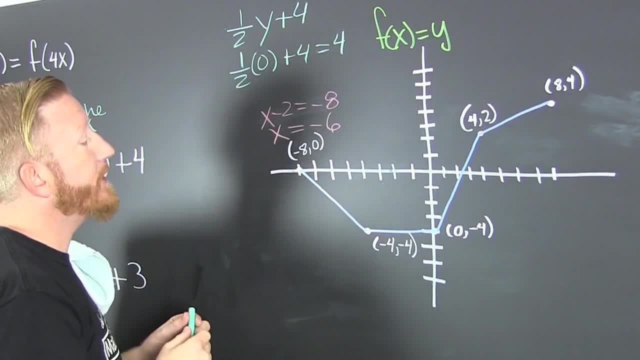 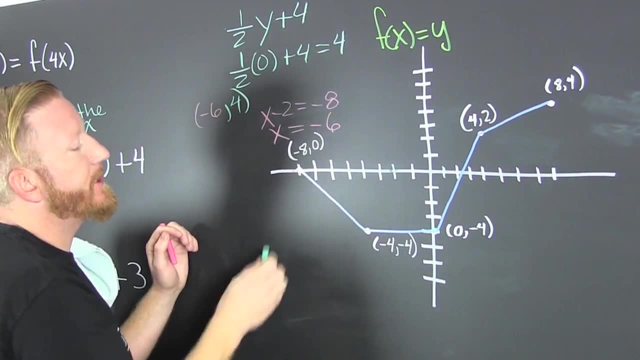 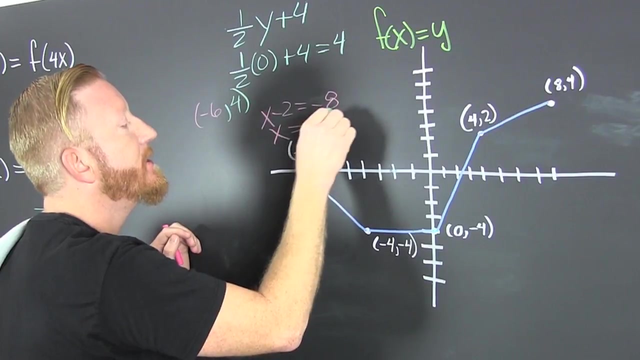 to a 4.. So my new point is going to be minus 6 and 4.. Let's look at that: 1,, 2,, 3,, 4,, 5,, 6, and 4.. There it is. Should have had another. 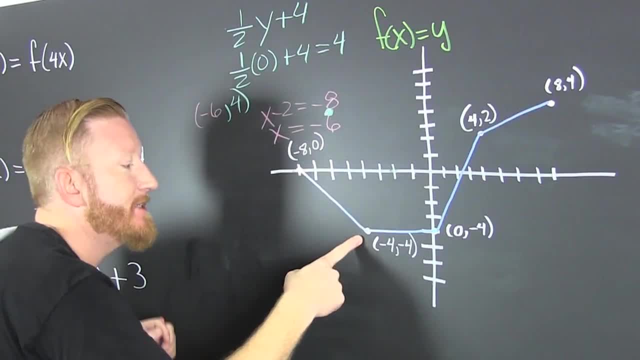 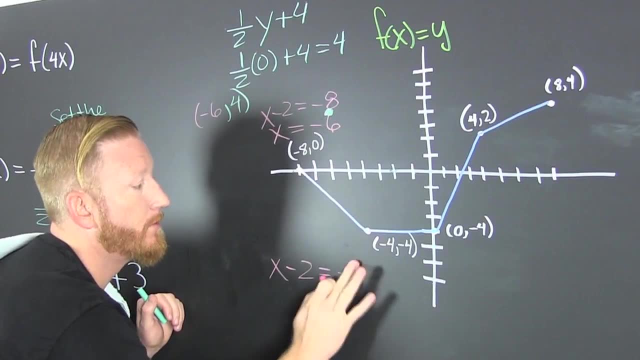 It's a different color, but here we are. Now let's translate this one That says: x minus 2 is equal to a minus 4.. Am I changing? x? That's equal to a minus 4.. So our new x. 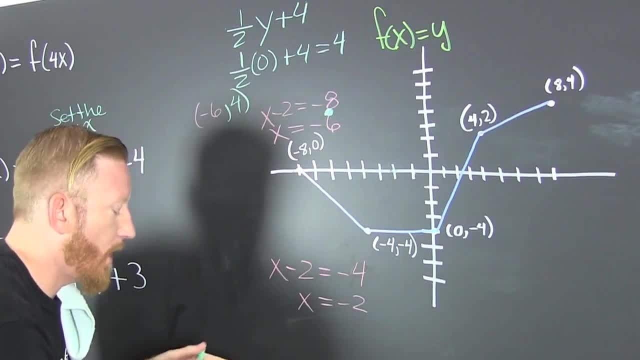 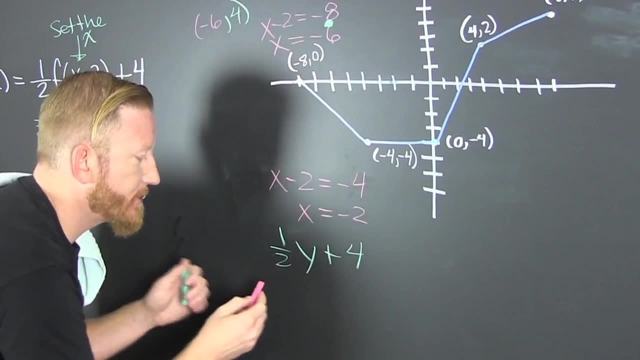 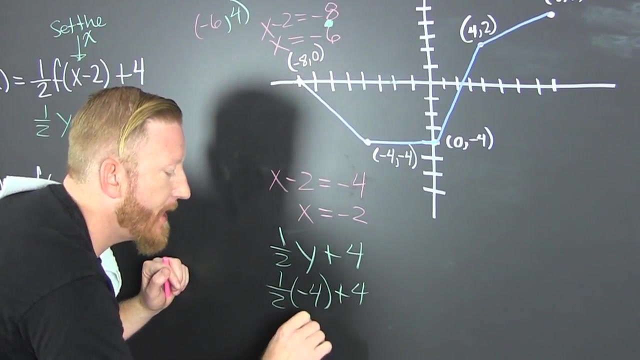 is going to be a minus 2.. What's our y? 1 half y plus 4.. Our y is a minus 4, so that's 1 half y plus 4.. 1 half y plus 4 is equal to a minus 4 plus 4.. Minus 2 plus 4 is 2.. So our new point is: 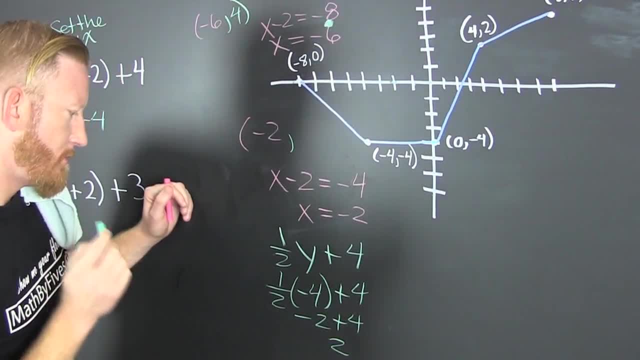 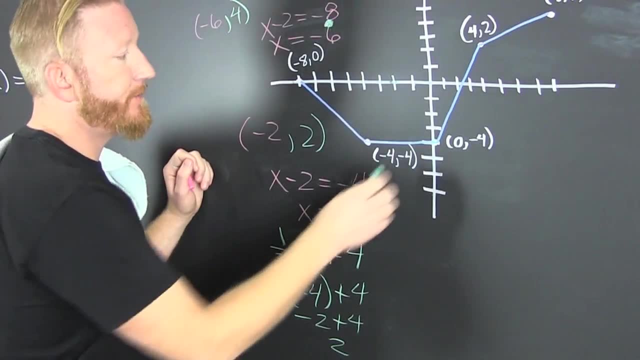 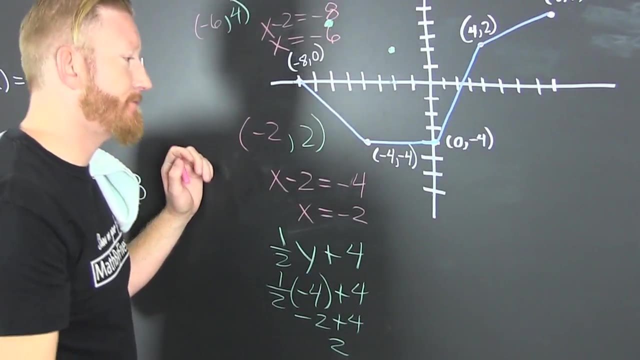 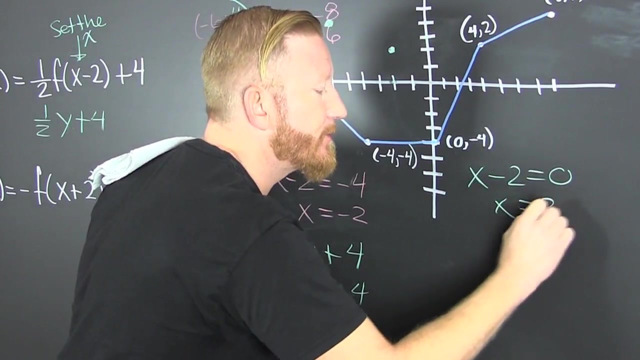 minus 2 and minus plus 4, 2.. Sure, This science got me all goofy there. So then, minus 2 and 2.. When we're making this translation- All right, Let's translate this point- We're going to have a new point. I've got x minus 2 is equal to 0. So then x is equal to 2.. Now 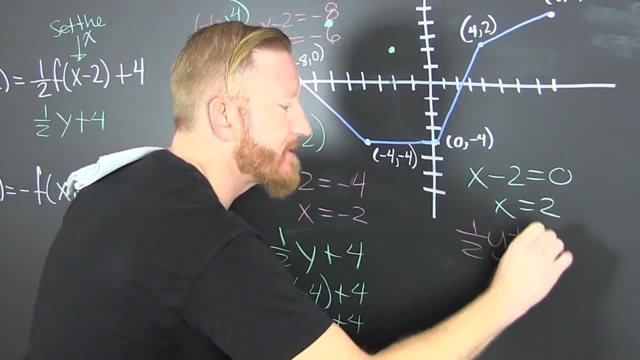 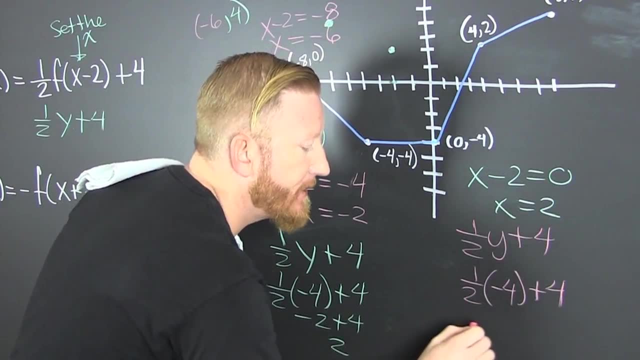 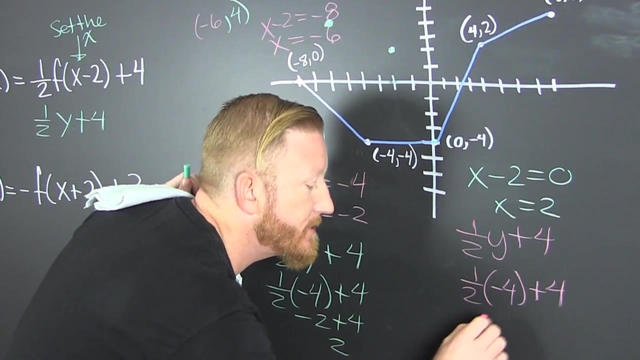 I have 1 half y plus 4, whatever y was, That's 1 half a minus 4 plus a 4.. Wait, wait, wait. Certainly it is because they have the same y value, That's a 2.. So our new point is 2,. 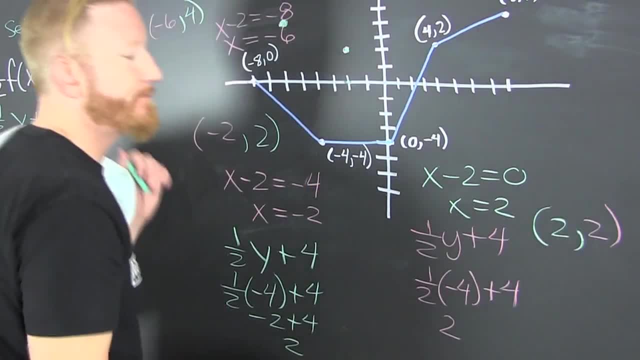 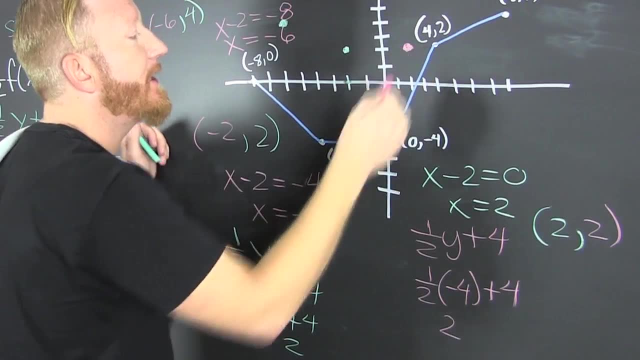 2., 2, 2.. What is a ballerina wear? This is 2 and 2.. That's our new point, right there. Now we're translating that guy right there. So x minus 2 is equal to 4.. And x is equal to. 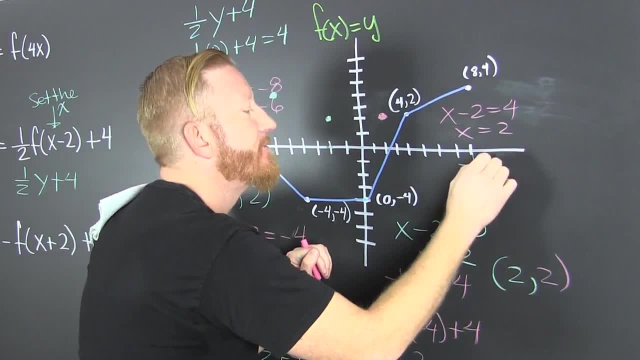 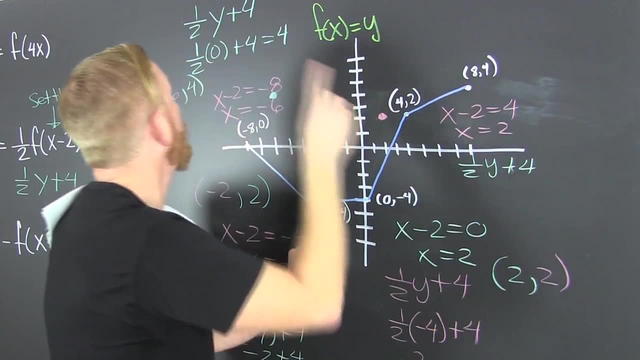 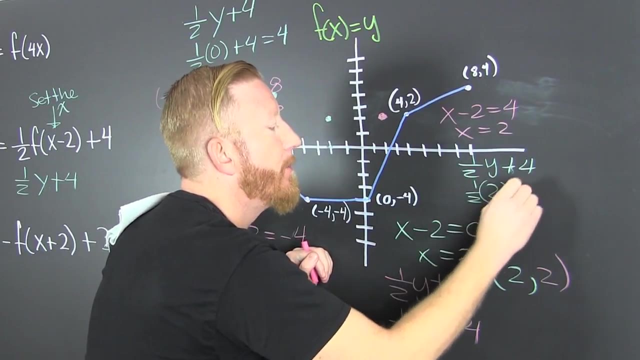 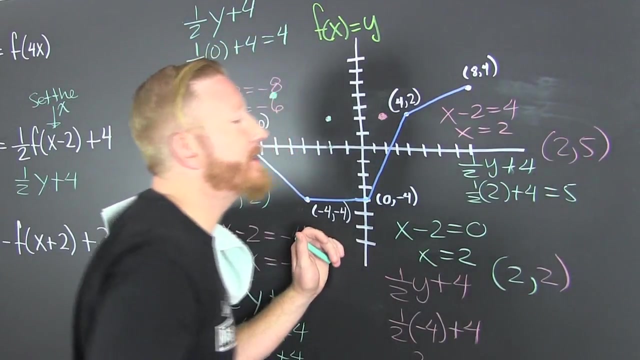 2.. That's our new x value: 1 half y plus 4.. 1 half y plus 4 is what we're using to translate that. what's our y? It's 2.. So that's 1 half 2 plus 4 is 5.. So our new point is 2, 5.. I'm going to work. 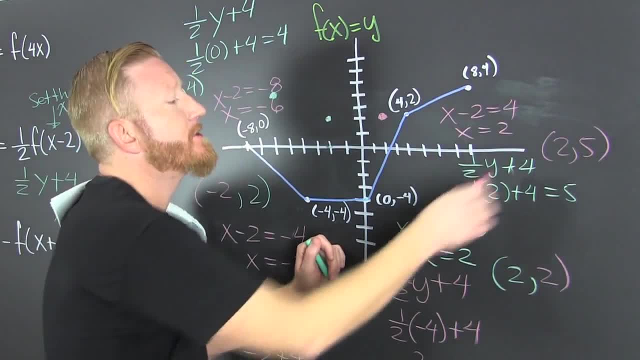 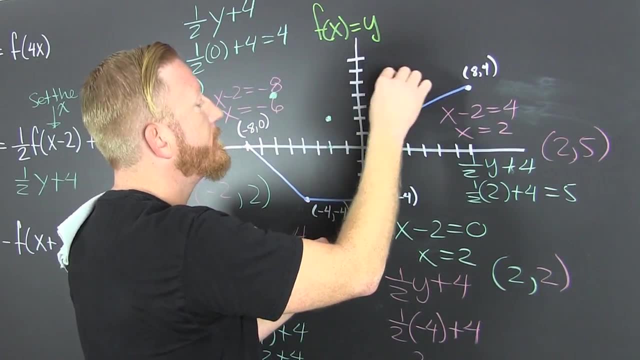 these out ahead of time. If I made a mistake there, comment down below. So then here we go. That's a 2 and 1, 2, 3, 4, 5.. Boom, Well, that ain't right, It was. what are we translating? 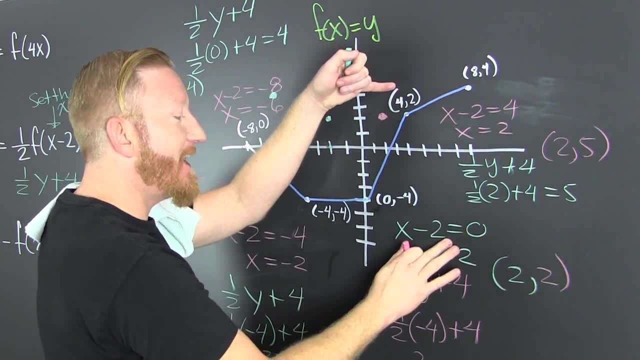 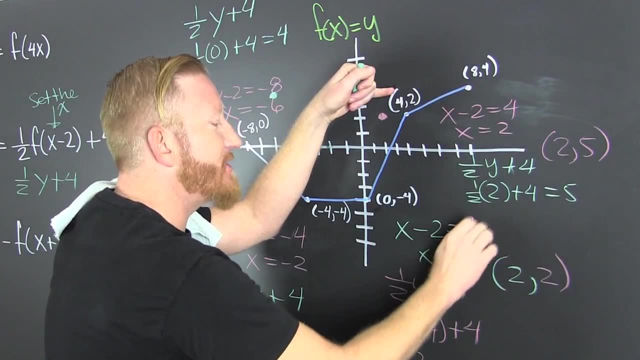 This one, No, this one. Oh, look at that, I caught it, I caught it, I caught it. Yeah, Don't, don't, don't freaking. No, no, that should have been a 4. Yeah, sure, Because. 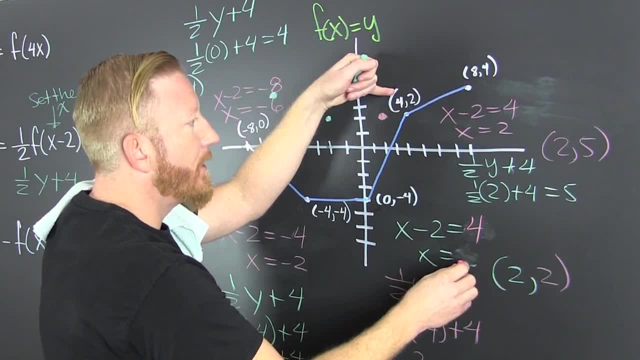 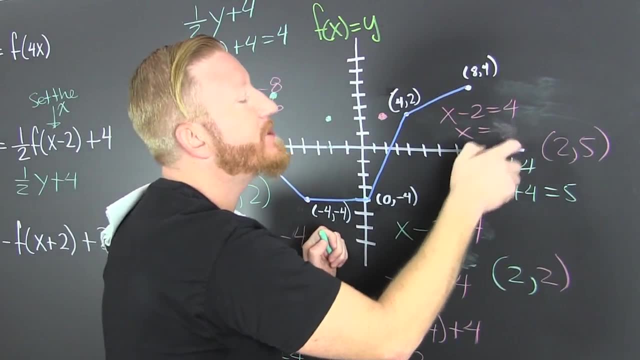 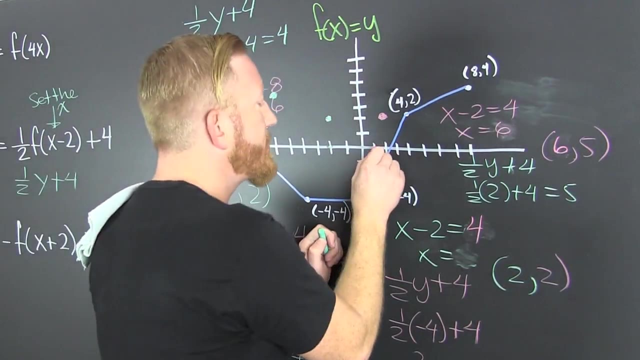 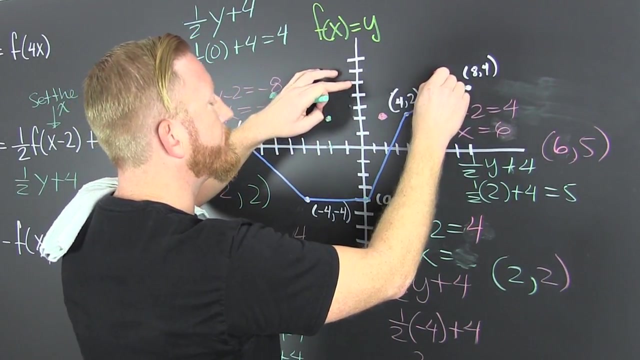 we were translating that x, then This turns out to be a o up there. Ignore that This was right. That was not 6. Boom, That's a 6. Boom. You were so happy with your key. So then this is 1, 2, 3, 4, 5, 6 and 5.. 1, 2, 3, 4, 5. Boom. Now I'm on tilt because I 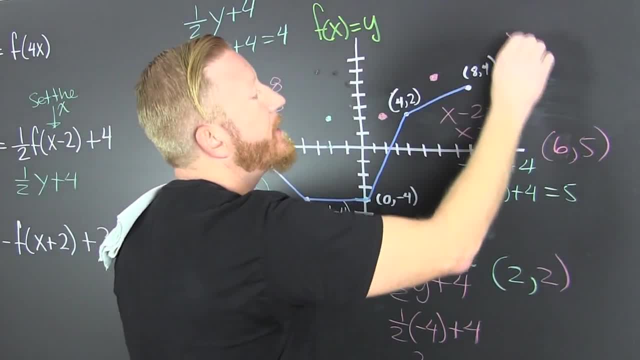 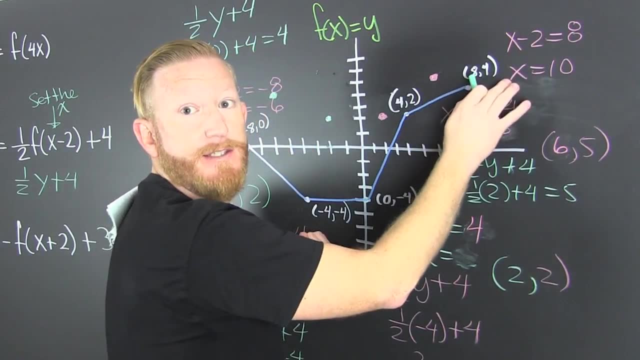 don't think I have enough ticks for that last one. Let's translate that x minus 2 is 8. Great, So then x is equal to 10.. Then we're looking at: can you see this? Yeah, you're. 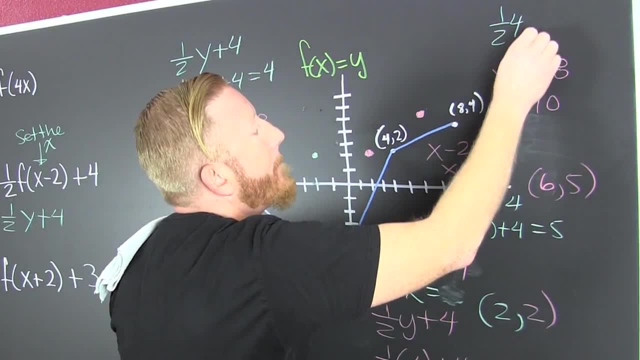 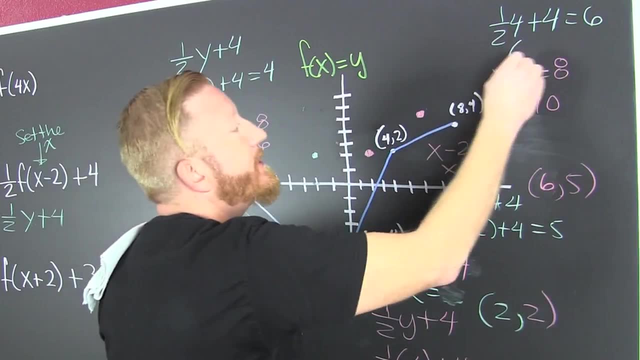 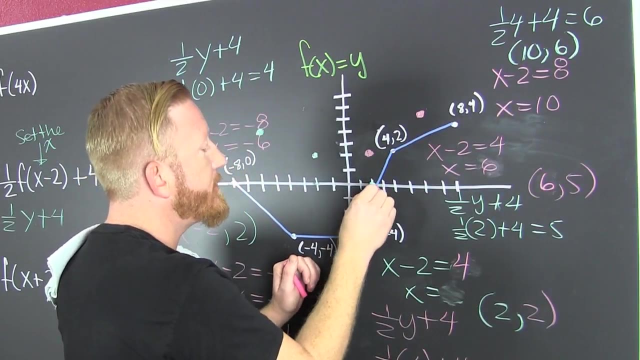 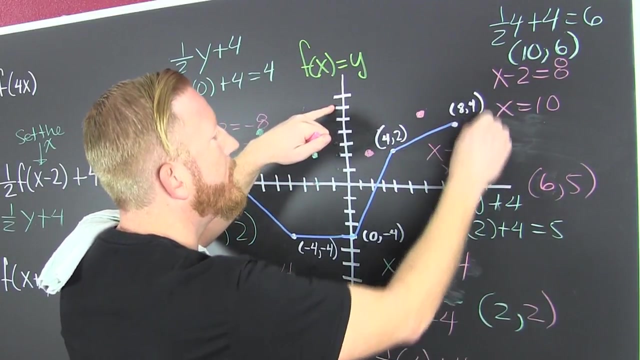 good, So then 1 half, 4 plus 4.. So that's 2,, that's 6.. Yeah, So then our new point. there is 10 and 6.. So then 10 and 6.. 1,, 2,, 3,, 4,, 5,, 6,, 7,, 8,, 9,, 10 and 6.. 1,, 2,, 3,, 4,, 5, 6.. Boom, So if we're translating, 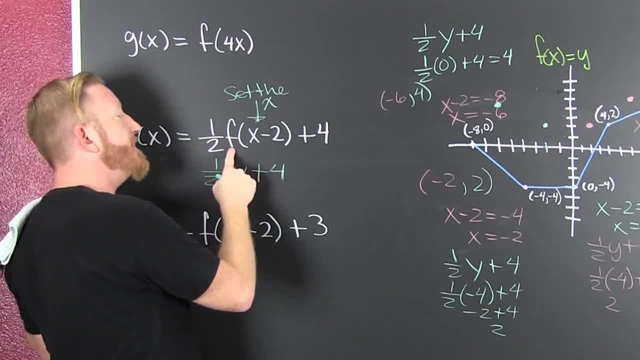 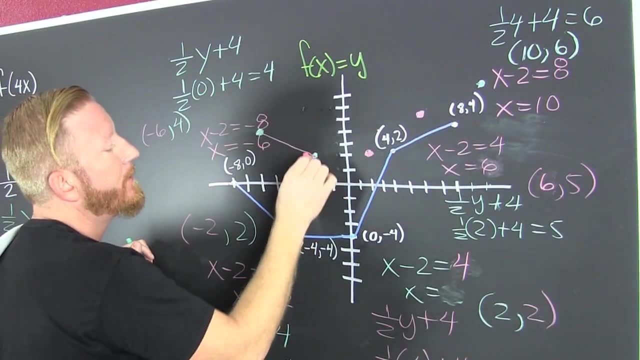 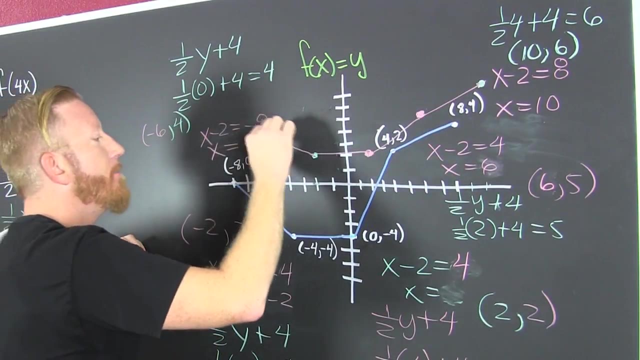 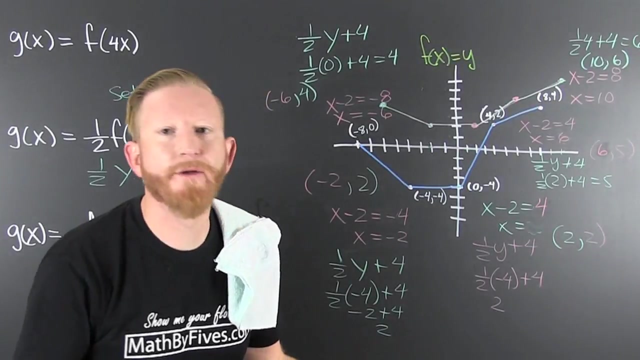 this g of x, which is 1 half of the previous f of x, shifted right to And up, 4, it's going to look like this guy: Boom, Boom, Boom, Boom. Yeah, It has the same basic shape, but it's squished, shifted and shifted again. One more. This time we're. 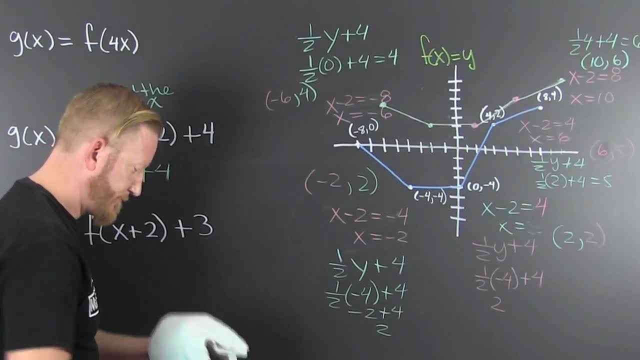 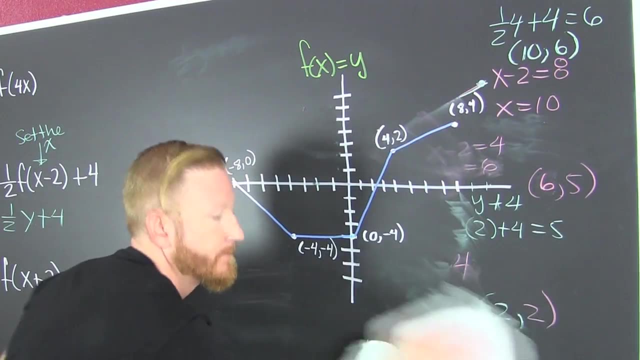 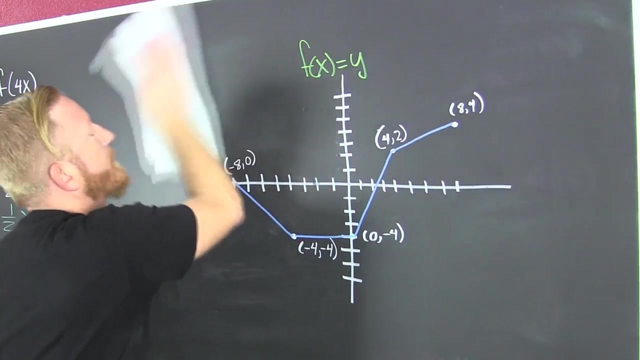 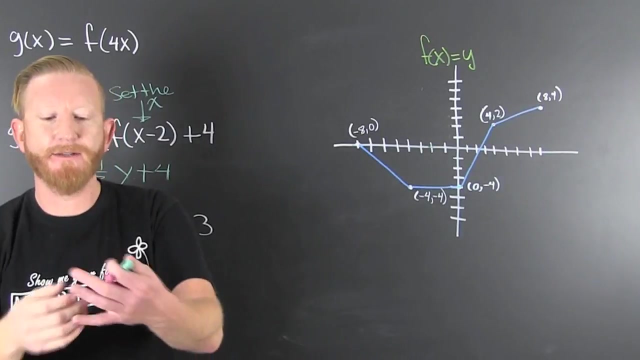 not going to find all those points. Boom, Boom, Boom, Boom. Pardon me, I'm clearing the table For the table dancers. Oh my gosh, Drake, We're trying to do right and cover everything. One more: Ready, Ready, Ready. 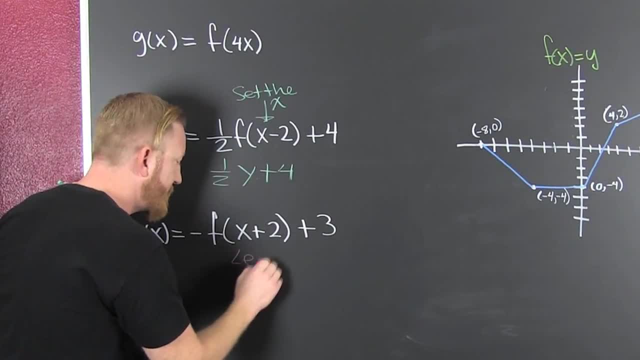 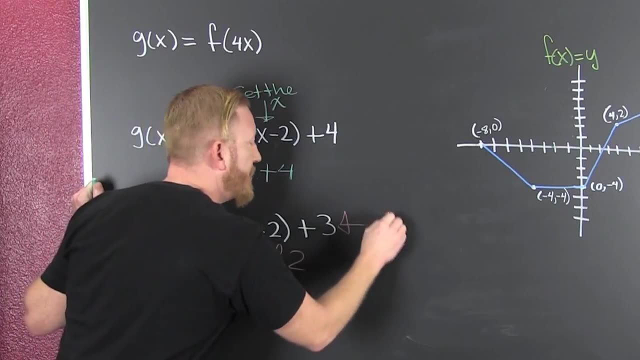 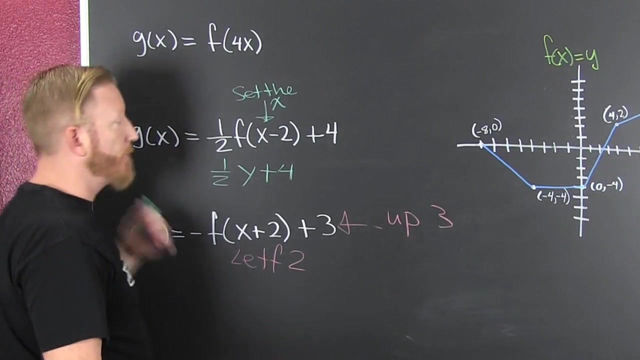 Ready? Oh boy, That's left. 2. Because it goes opposite the way you think That's up. 3. flip it. That takes all your y's and flip it. So, so, so, so, so. so We're going to take our y and 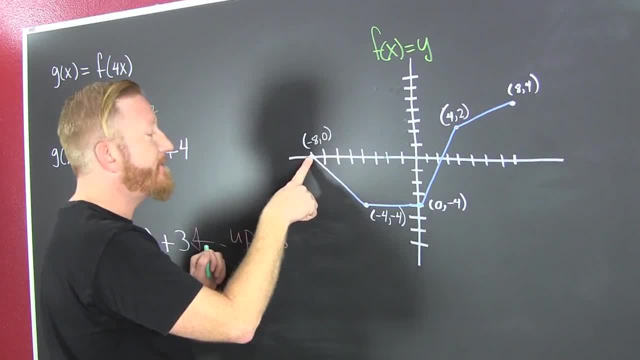 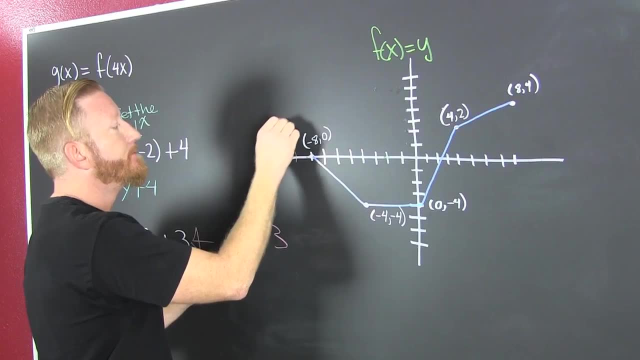 flip it, but it's at zero. so we're going to stay there And then we're going to shift. that left. two units: One, two, boom. And then we're going to go up. three units: One, two, three. We put a dot, Boom. 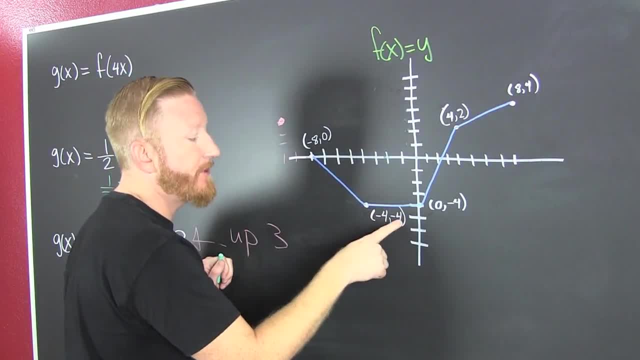 That's going to be our new point for there. Now we're going to flip this, We're going to flip the y value, so the y value is going to be four. Yeah, that's the flip on the outside, And then we move. 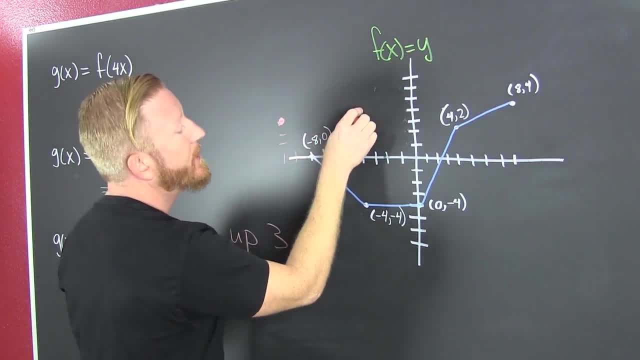 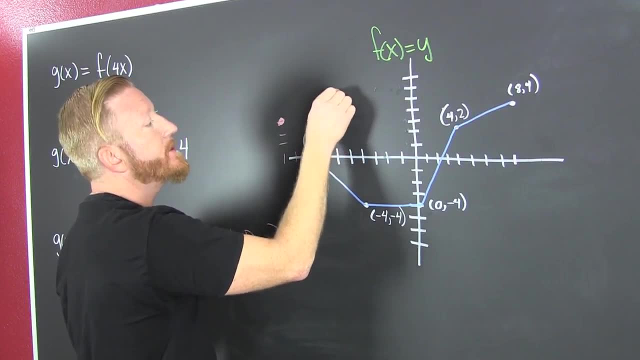 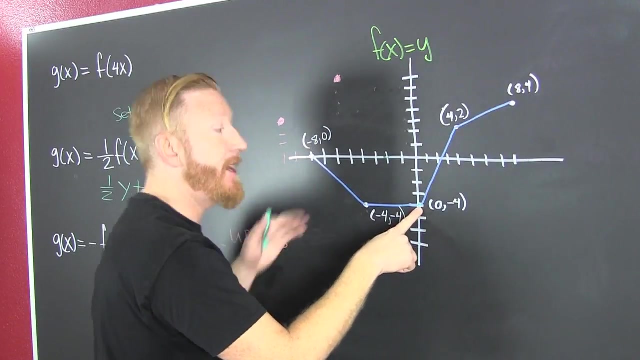 left two units and up three units. So from this point we go left one, two and up three. One, two, three, Boom, And that's going to be that point. Then this one, we flip it across the. 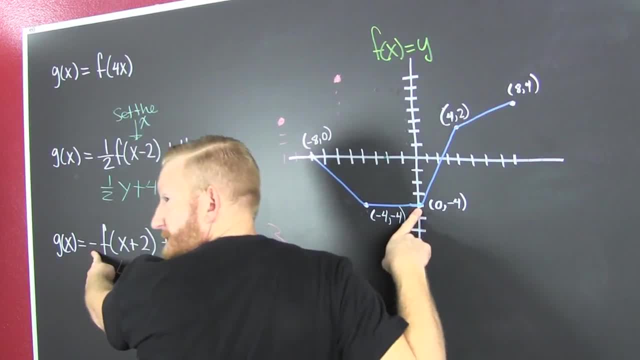 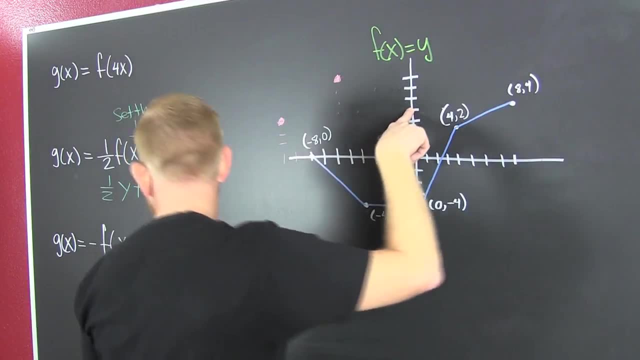 x-axis, because it's the opposite of y. That's what the minus does over there. It takes the opposite of y. So we take the opposite of y. That's going to be four, All right, And then we shift that left. 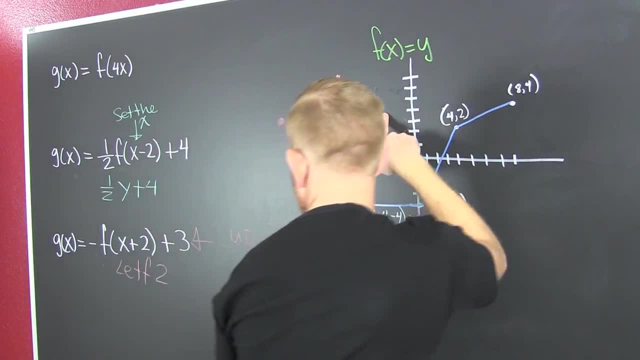 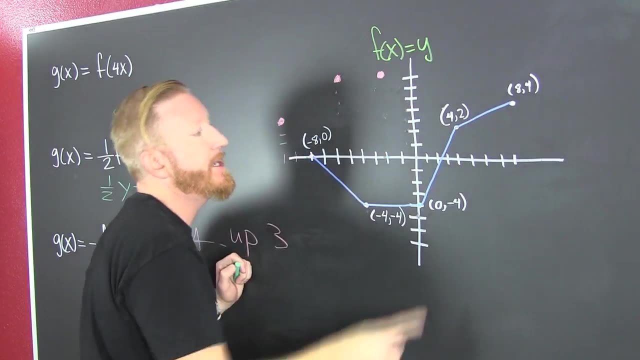 two, One, two, And then we shift that up three, Up three, One, two, three, Boom, And that's our next point. Okay, Now this one, we flip it. It was a positive two, Now it's a negative two. 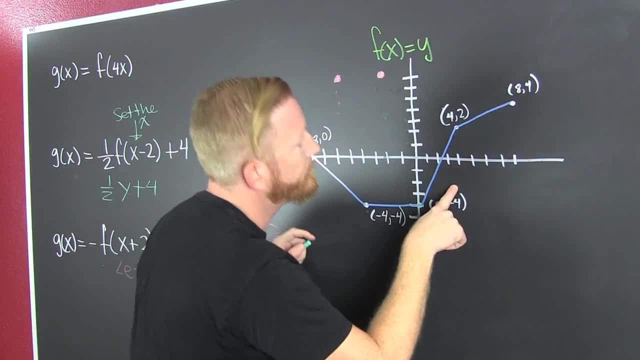 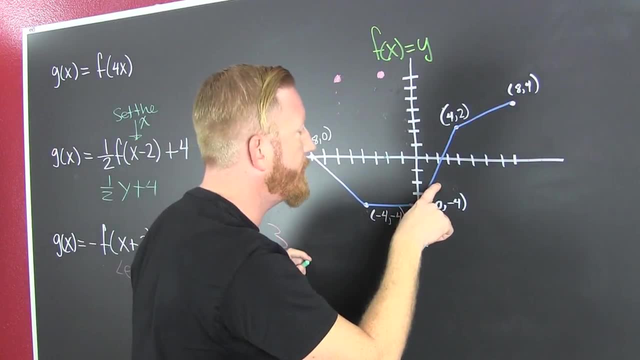 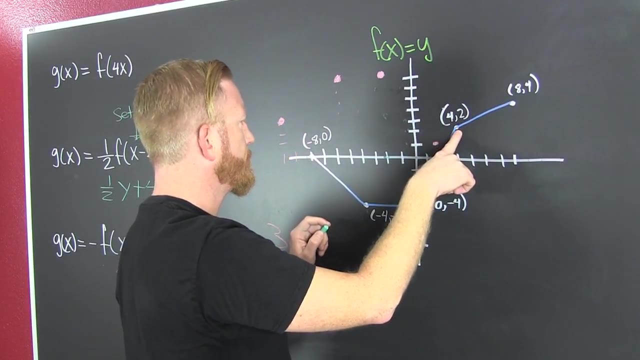 Flip and move. So we flipped it. Then we go left, two, Left, two, Boom. And then we go up three, Up three. So we go up three from there. One, two, three, Boom, Okay, And that's that new point. Yeah, We've got four points down. One left to go Flip it, It was y is. 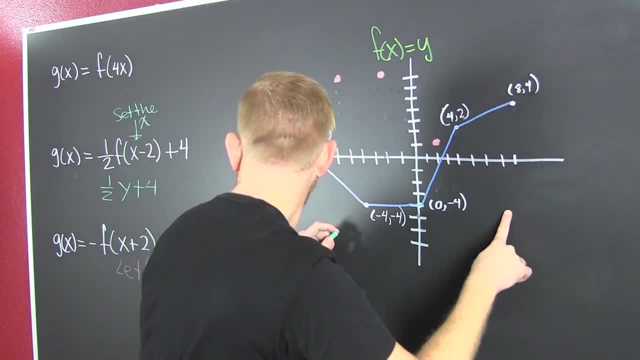 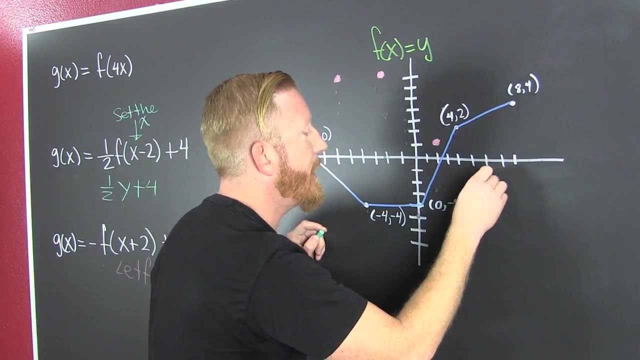 equal to four. Now it's y is equal to minus four. And then we go left two units, One, two, And then we go up three units. So then we go up three units And then bam, that's our new point. We. 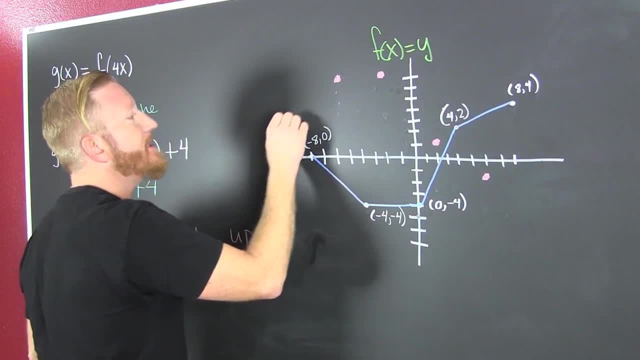 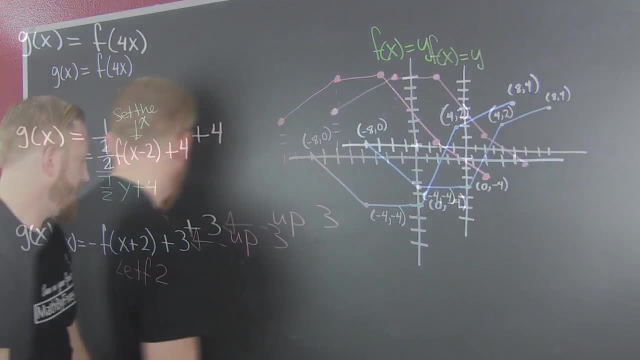 could check them all algebraically, But if we were looking at this, see Boom Boom, Boom Boom- It's our original graph, Flipped upside down, Shifted, left two Boom Boom Boom And up three.